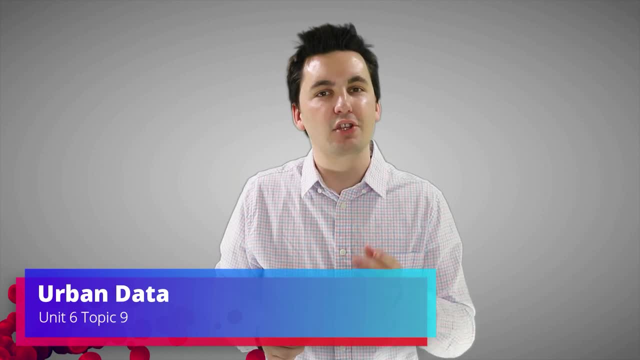 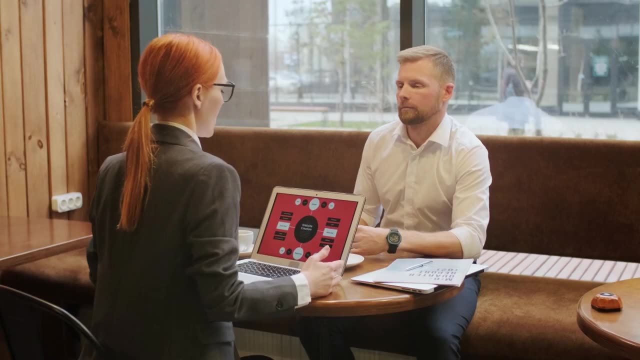 We're going to be talking about how governments make their decisions and how they can use qualitative and also quantitative data to make sure they're making decisions that benefit society as a whole. Qualitative data is often gathered through surveys and polls. This data is subjective and is up for discussion. 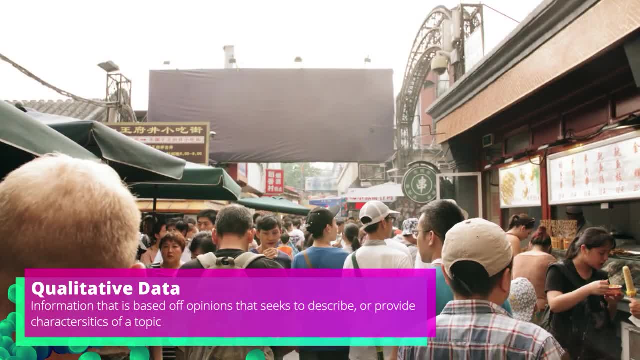 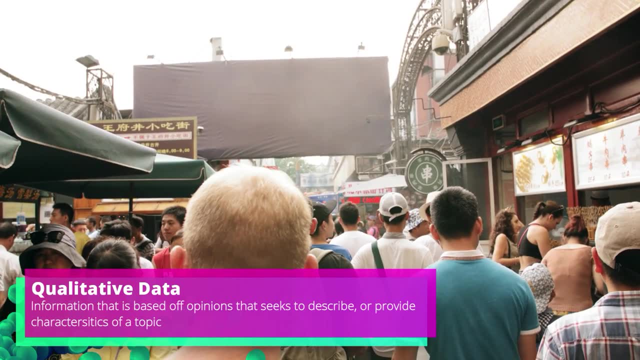 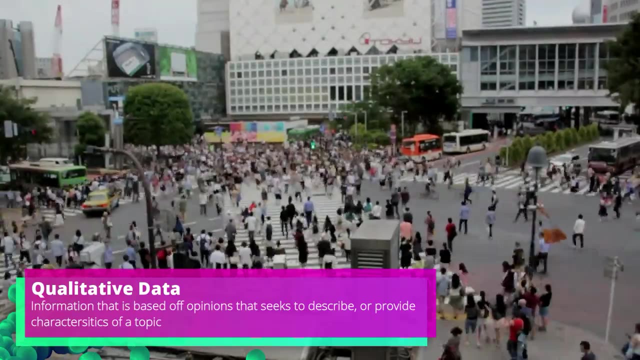 The data is often gathered through open-ended questions. This data can help cities better determine what the residents need and what they want from their city officials. Cities will collect information on the quality of the schools, hospitals, police, fire response and people's opinions on new parks, public transportation. 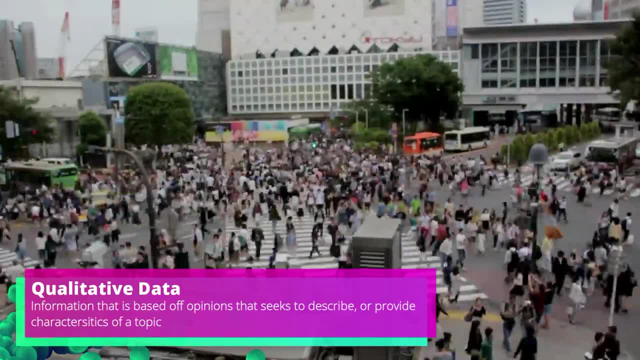 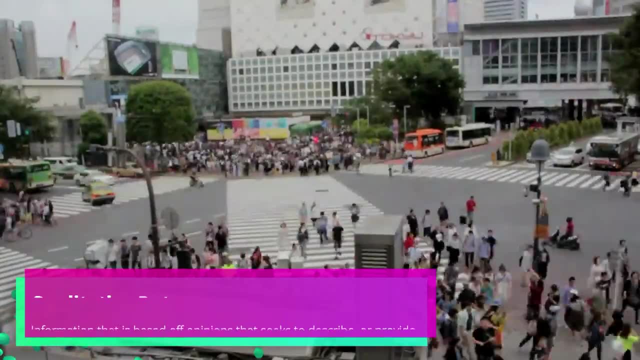 or even just data on traffic and the day-to-day interactions people have within city limits, to better understand how they can make a city that works for the residents that reside within it. Quantitative data, on the other hand, is often in number form and is not up for discussion. 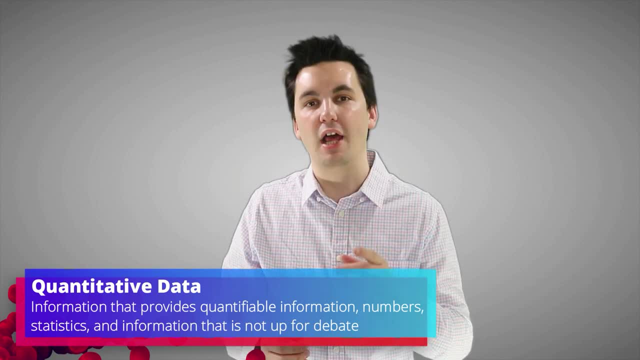 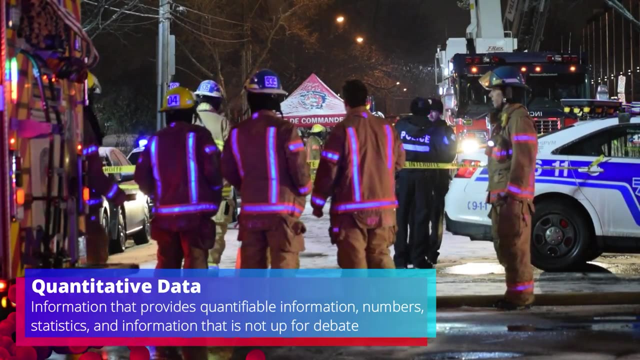 This data can be replicated in studies and will often help cities focus on specific issues. For example, city officials could look at the amount of accidents happening at certain intersections to see if a road needs to be rerouted or if the city should put in a stop sign or stoplight, or maybe even a roundabout to block an road. 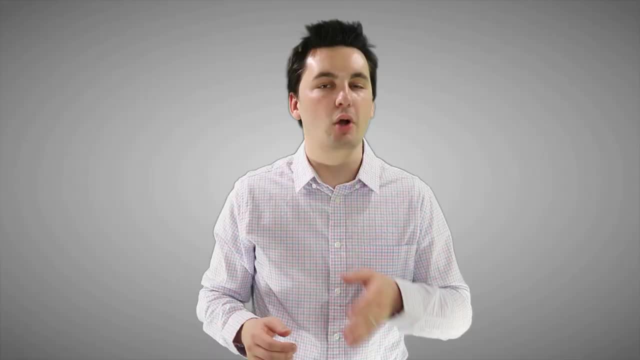 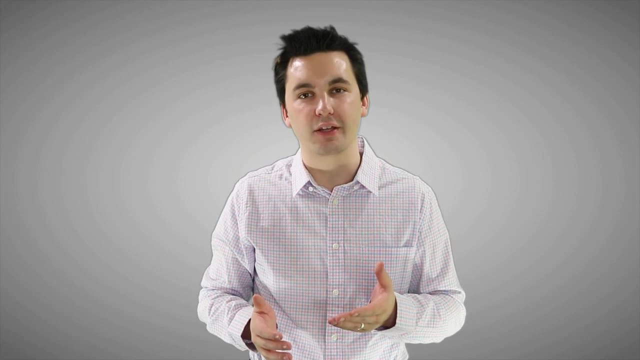 This data is often collected through polls. It is critical data to better understand how cities can make decisions that make sense for the residents that reside within it, help reduce the traffic. Most of the time, quantitative data is going to be found through quantitative research or by looking at things like the census or also surveys. We can also see that 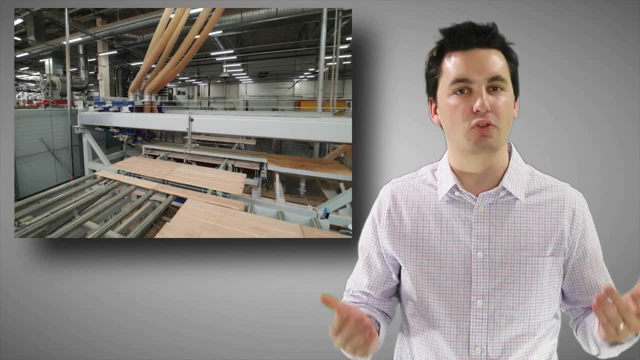 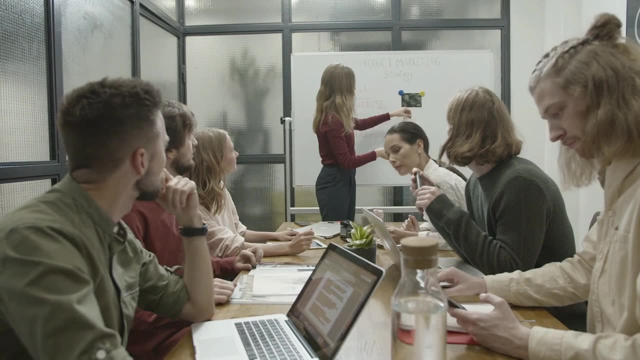 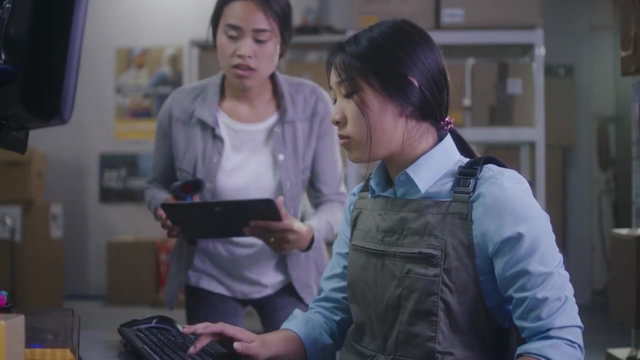 the private sector uses both quantitative and qualitative data as well. Businesses use surveys to collect qualitative data to understand the needs and wants of their customers, to allow them to understand what their customers experience are with their stores and also understand what products they want in the future. They also use quantitative data to better understand the 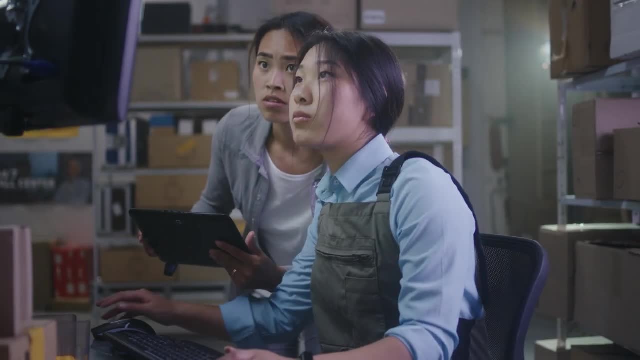 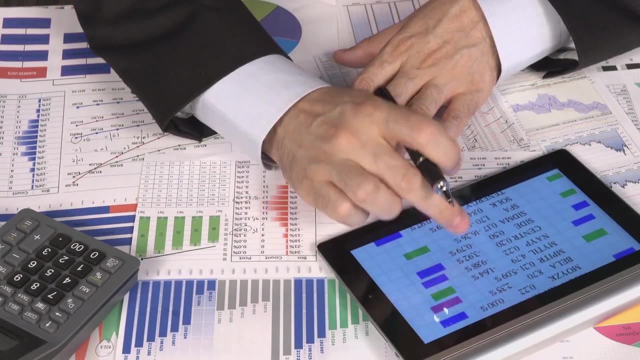 threshold of an area. To look at the demographic data of a region can help a business better determine if that geographic area is a place they should expand their business in and if there is enough money and people to be able to support their store. When the private sector and the 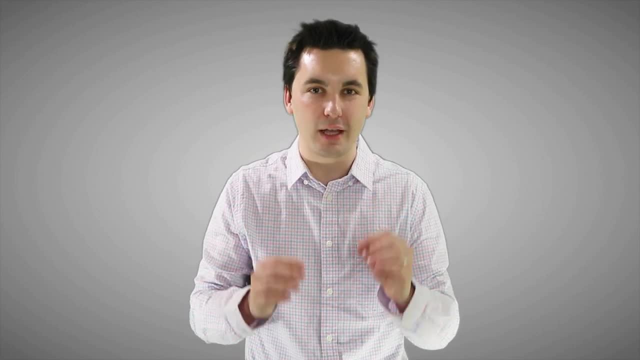 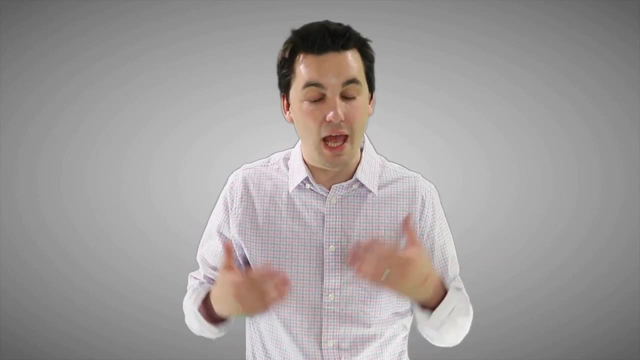 public sector. both use qualitative and quantitative data correctly, they can make a better city and a better society for all people. It'll allow them to use their resources efficiently and maximize their productivity. All of this will help raise the standard of living and reduce frustration in the city.